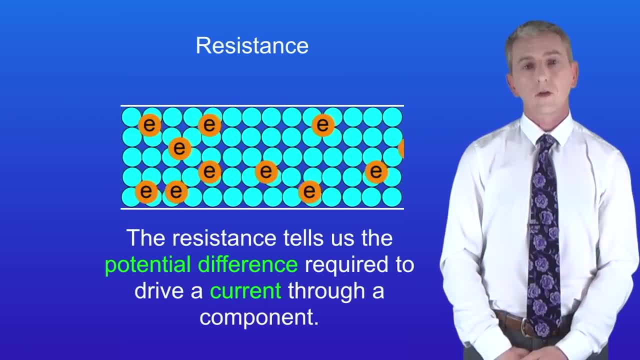 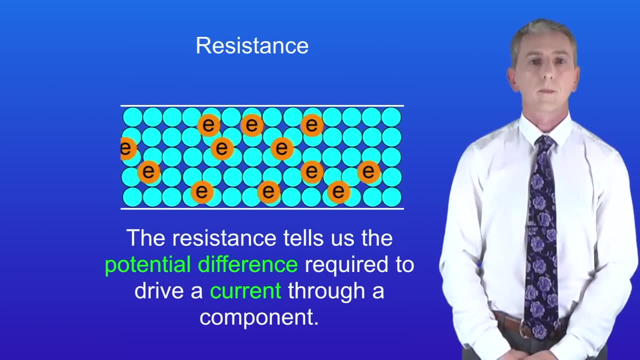 The resistance simply tells us the potential difference required to drive a current through a component, In other words, how much energy is required to push a coulomb of charge through. I'm showing you here two circuits containing different lamps. A current of one ampere is moving. 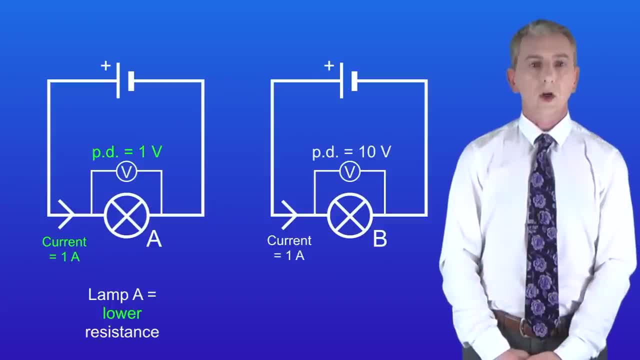 through both circuits. In lamp A the current is being driven by a potential difference of only one volt. This tells us that only a small amount of energy is required to drive the current through this lamp. So lamp A is a low resistance lamp. In lamp B, the current's being driven by 10 volts. 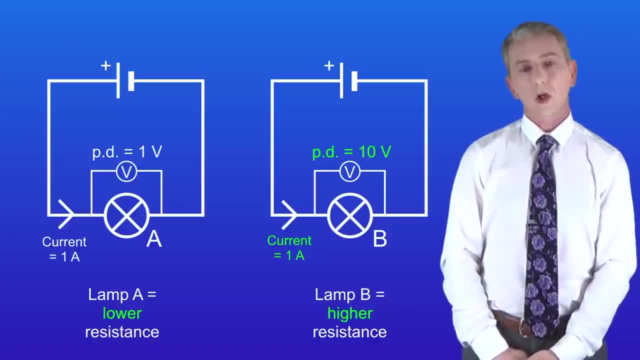 This means that a relatively large amount of energy is needed to drive the current through lamp B. Therefore, lamp B has a higher resistance than lamp A. It simply takes more energy to drive the current through lamp B. So can you see that the idea of resistance is actually fairly straightforward. 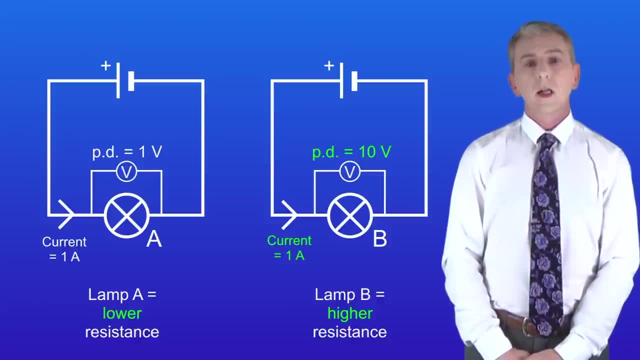 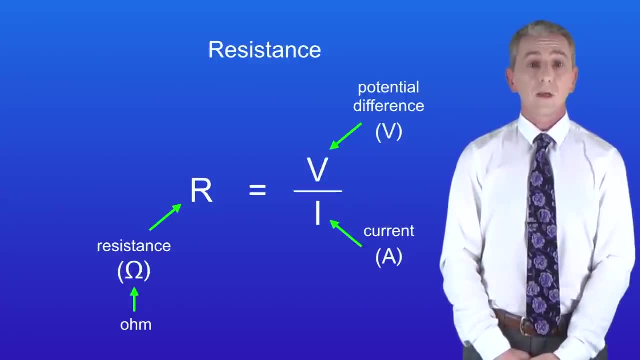 Now you could be asked to calculate the resistance of a component. It's easy to do this. we simply use this equation: The resistance equals the potential difference in volts divided by the current in amperes. The unit for resistance is the ohm, and you could be asked: 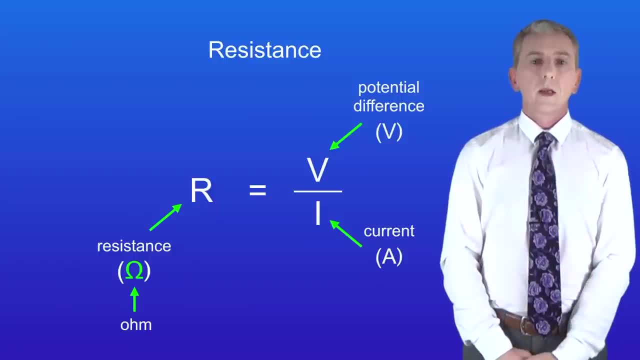 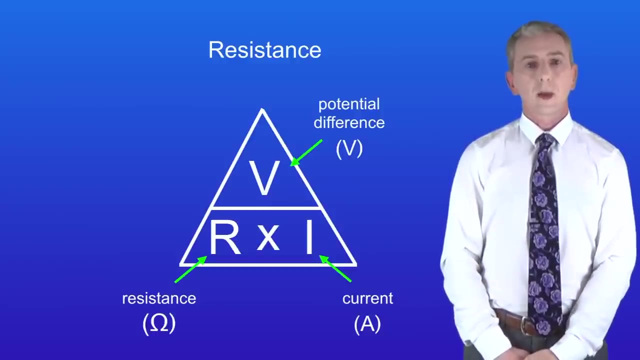 that. Here's the symbol for the ohm. You're not given this equation in the exam, so you need to learn it. Many students prefer to use a triangle for equations, So here's the triangle angle for this equation. So we're going to work out the resistance of the two lamps that we saw. 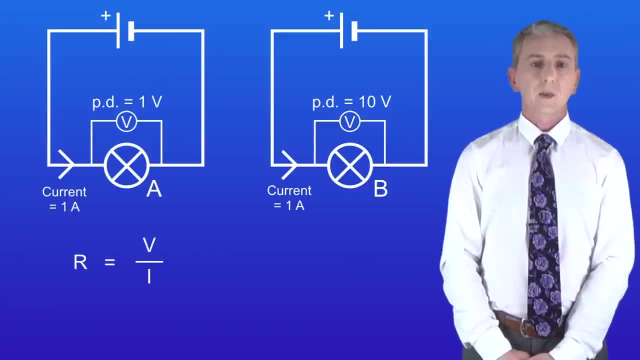 before. Lamp A has a current of 1 ampere and a potential difference of 1 volt. Putting these into the equation gives a resistance of 1 ohm. Lamp B also has a current of 1 ampere, but this has a potential difference of 10 volts. Putting these numbers into the equation gives us a 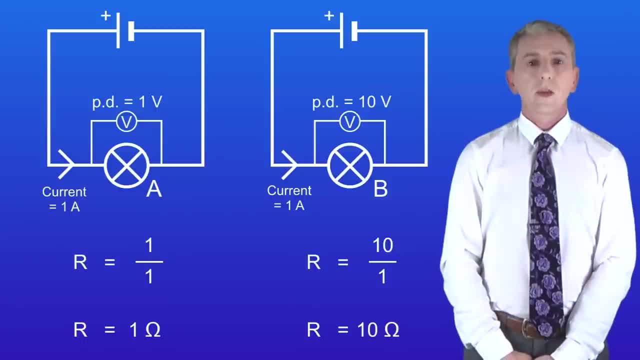 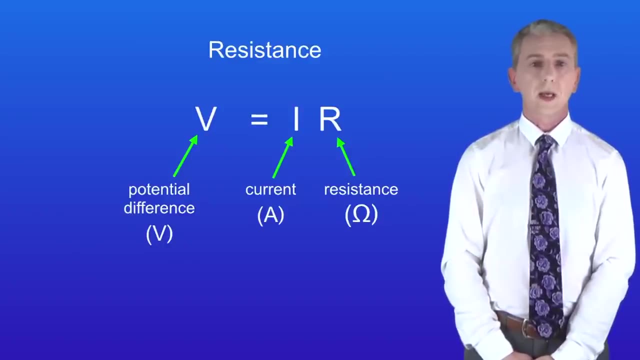 resistance for lamp B of 10 ohms. Now in the exam you could be asked to work out the potential difference needed to produce a certain current. To do that we need to rearrange the equation for resistance like this: The potential difference in volts equals the current in amperes multiplied. 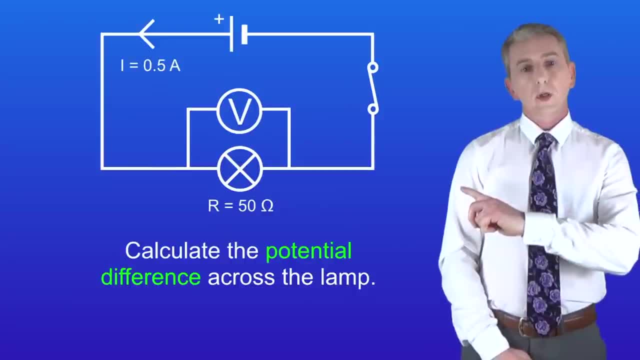 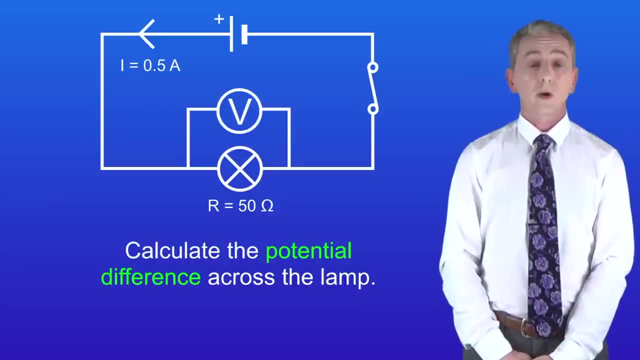 by the resistance in ohms. Here's a typical question: Calculate the potential difference across the lamp. We can see that the current is 0.5 amperes and the resistance of the lamp is 50 ohms. So to calculate the potential difference. 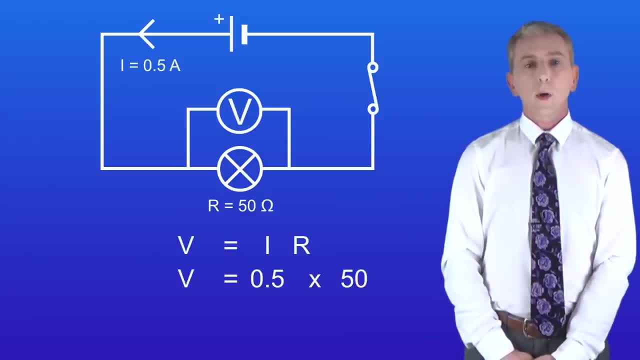 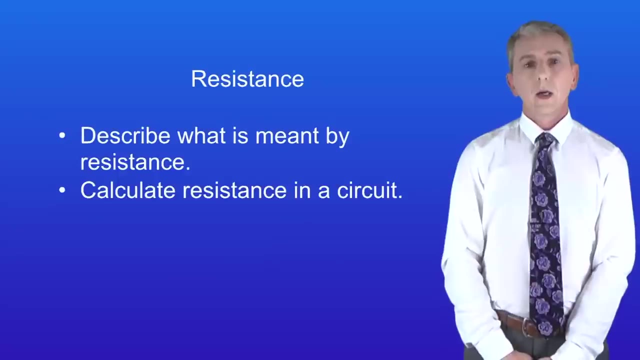 we need to calculate the potential difference across the lamp. We multiply the current by the resistance. 0.5 multiplied by 50 gives a potential difference of 25 volts across the lamp. Remember, you'll find plenty of questions on calculating resistance in my vision workbook, which you can get by clicking on the link above. Okay, so hopefully. 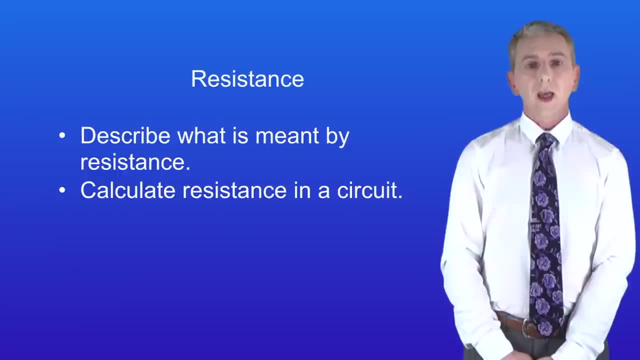 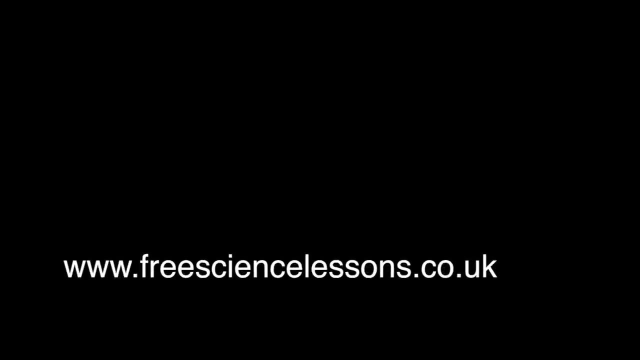 now you should be able to describe what's meant by resistance. You should then be able to calculate resistance in a circuit. Thank you so much for watching. I hope you enjoyed this video and I'll see you in the next one. 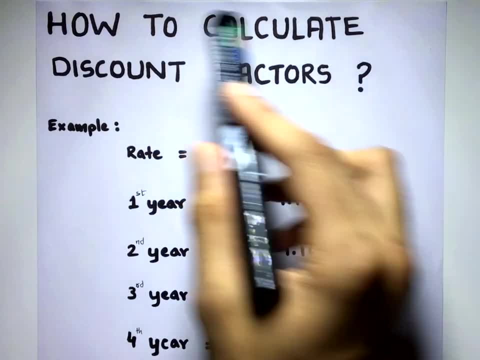 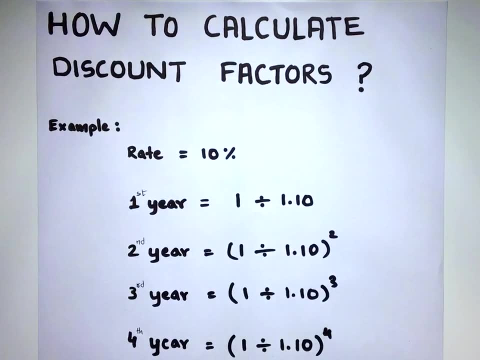 Hi everyone. Today we are going to understand how to calculate the discount factors for NPV or IRR calculation, and all when discounting tables are not provided in exam. See, it's really simple. Let's take an example. Let's say the rate is 10% and you want to calculate the discount factors. 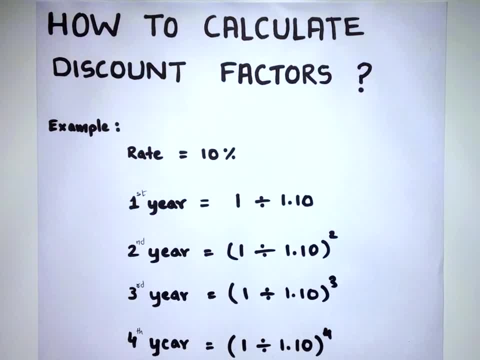 for four years after first year, second year, third year, fourth year. So see, the formula is really simple. What are you going to do? 10%, right? So you are going to take 1 divided by 1.10.. If it, 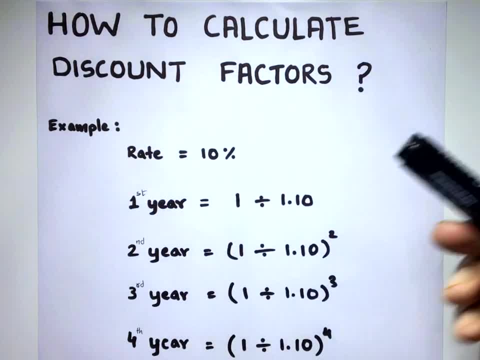 was 7%, 1 divided by 1.07.. If it was 6%, 1 divided by 1.06, like that, Okay, and then you are going to keep raising the power. Okay, for second year, raise the power to 2.. For the third year: raise the power. 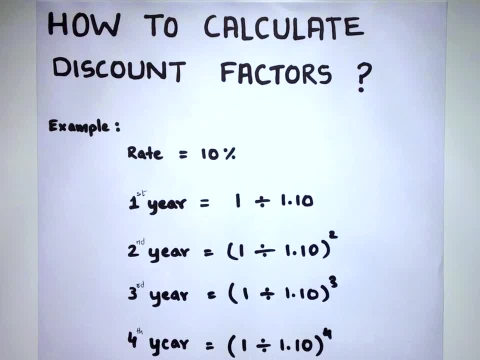 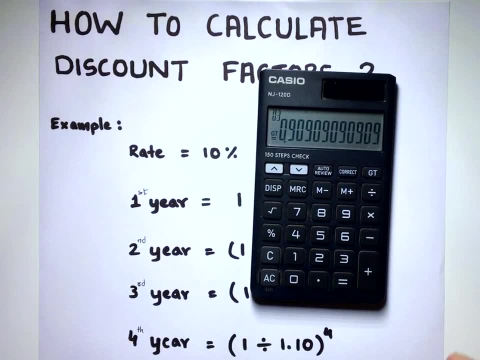 to 3.. For the fourth year, raise to the power to 4.. But now how will you do this in normal calculator? See, it's really simple. 1 divided by 1.10 is equal to discount factor after first year is equal to. 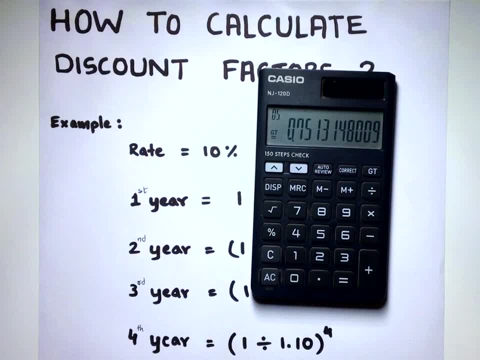 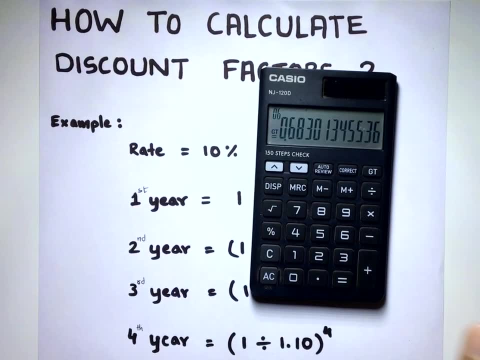 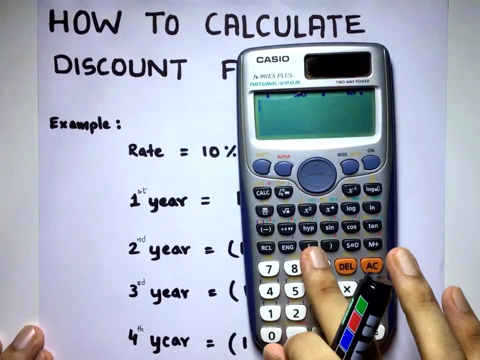 discount factor after second year is equal to discount factor After third year. Okay, you keep on doing this, Is that okay? One more time: discount factor after the fourth year. That's simple. Now, scientific calculator is also really easy because you know the formula. What are you going to do? See, let's just use the brackets first. 1 divided by 1.10.